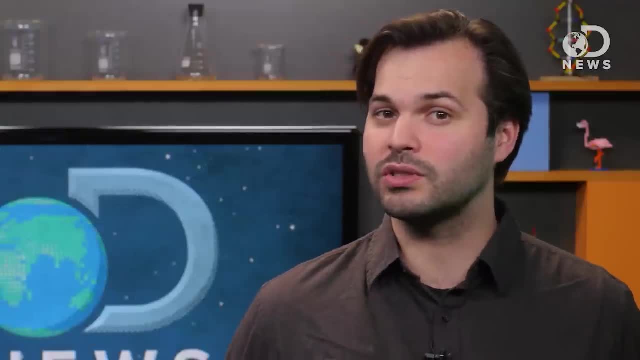 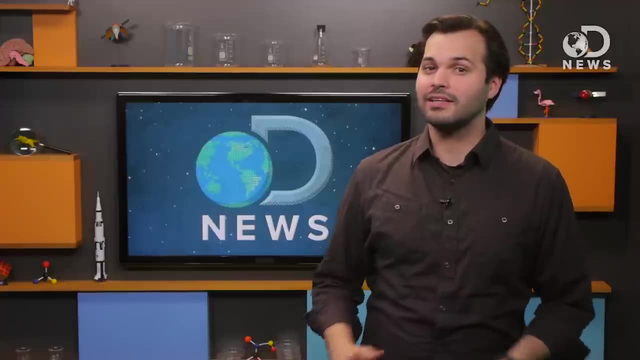 to keep the fly off their bodies. But by studying their visual system, scientists conclude the zebra's stripes seem to screw up the fly's vision. If they can't see to come in for a landing, then the fly will go bite some other animal. Nice Zebras aren't the only ones. 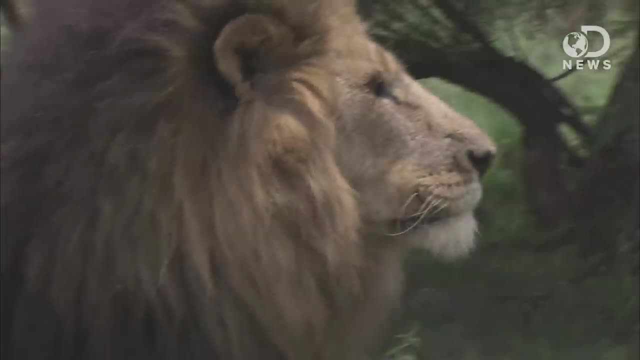 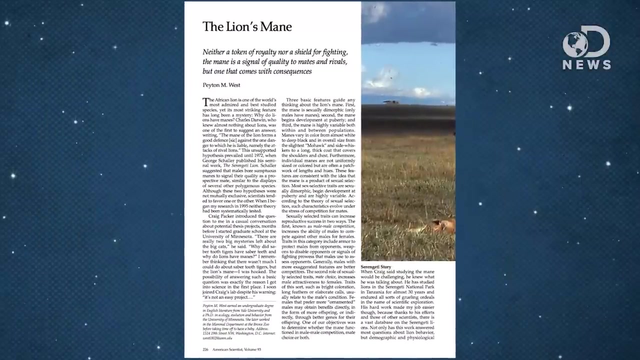 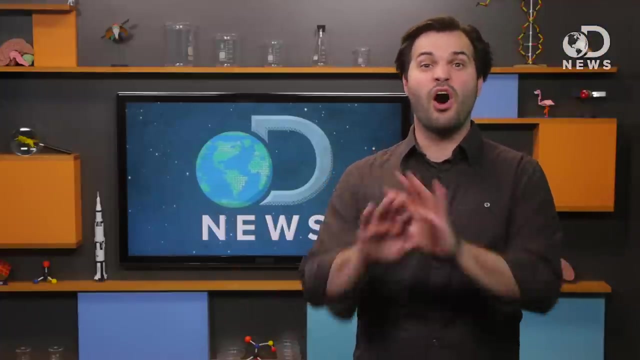 with this less-than-obvious adaptation. What do you think the lion's mane is for? Making it look big and awesome. American scientists published an article in 2005 detailing 30 years of lion study. Lions' manes aren't for intimidation. they aren't for protection. Based on ALL of their data, 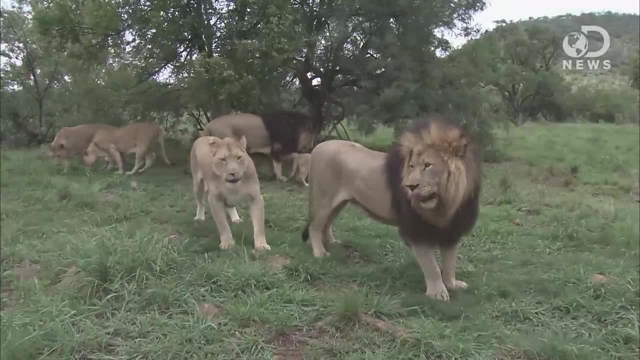 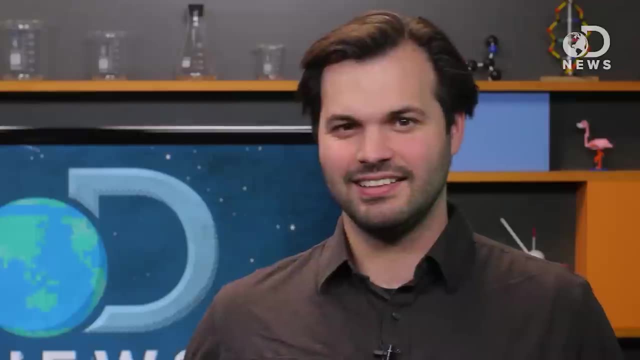 manes are for the ladies. Darker, larger manes indicate a well-fed lion, who is obviously good at hunting and has higher levels of testosterone, which is great for breeding. These aren't the only ways animals unexpectedly adapt to their surroundings. If you're. looking at giraffes, you'd probably figure, oh, they're not the only way they adapt to their surroundings, They're just a bunch of other animals. But if you're looking at a giraffe, you'd probably figure, oh, those trees are tall. 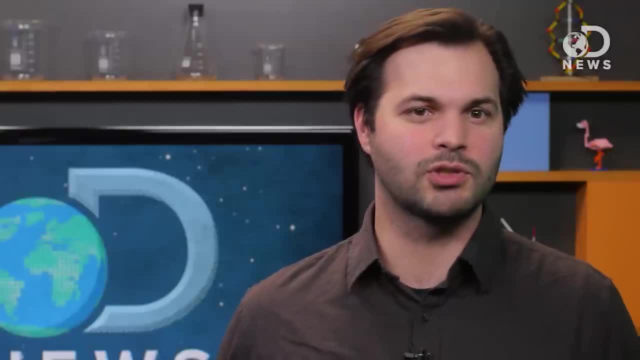 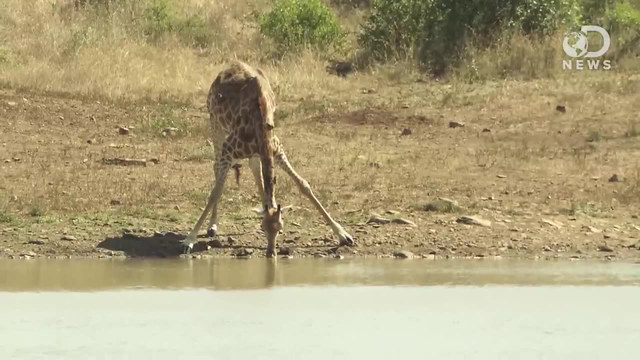 thus longer necks, right, Wrong again. Studying these animals, biologists guess the long neck has nothing to do with the height of their preferred food source, because it's extremely dangerous for a giraffe who needs to drink to bend over. Not to mention the neck is horrible for the giraffe's heart. 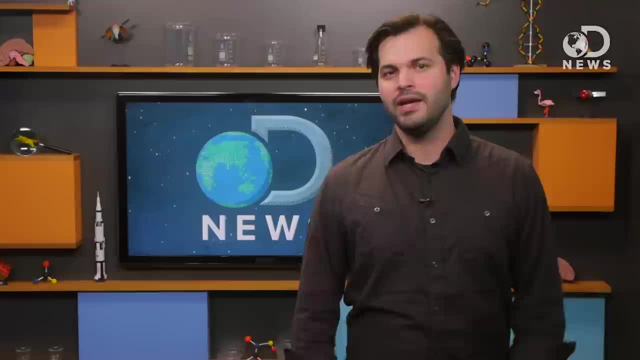 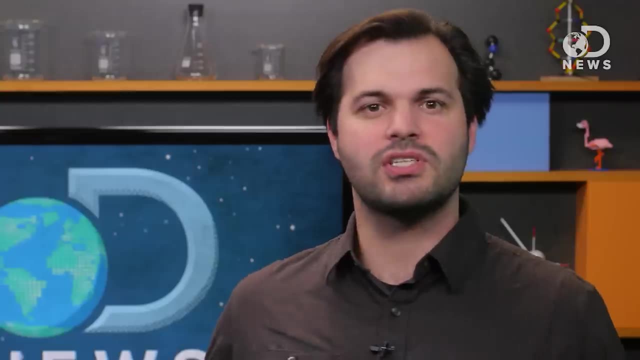 It has to work really hard to pump all that blood way up there. Instead, it may have started as an evolution for food, but giraffe's long necks are to compete for mates. Ever seen a giraffe fighting another giraffe? They whip their thick-skulled horned heads at other males. 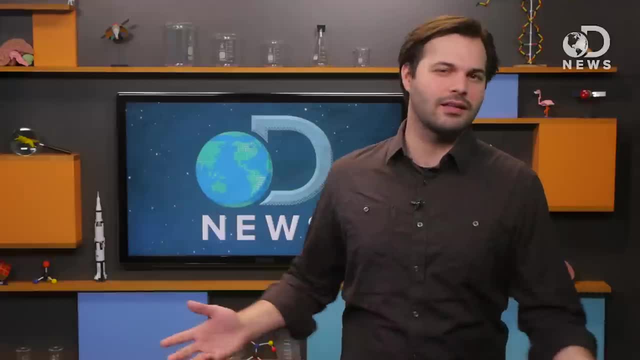 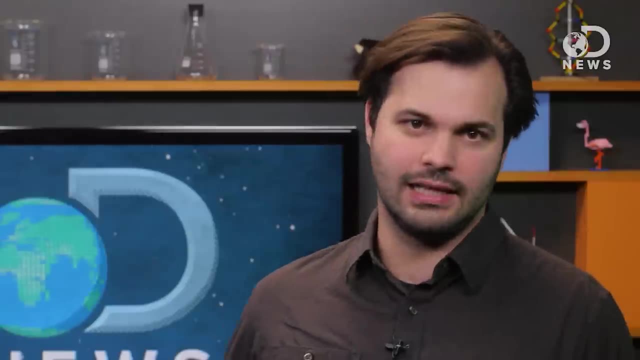 trying to fight for the right to party. Physics tell us this makes their head accelerate dramatically in comparison to the movement required at the base of their neck. That thing's deadly. Scientists are still studying the giraffe, but Uppsala University found that the necks 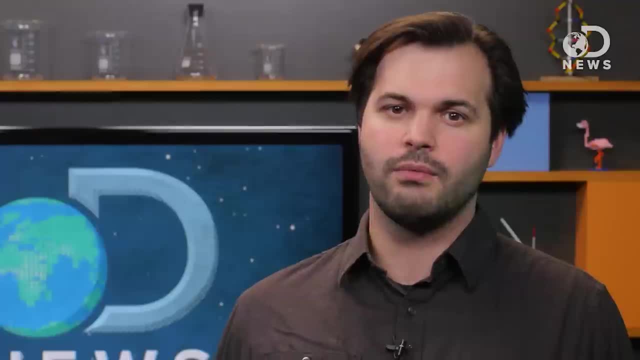 and skulls of male necks are longer and heavier than the females', which would support the neck for sex theory. I guess we'll have to put our neck on the line to go, for each other's necks Rock on like a duo. poor study.